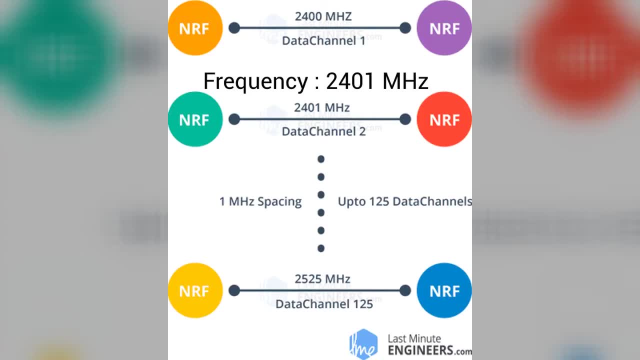 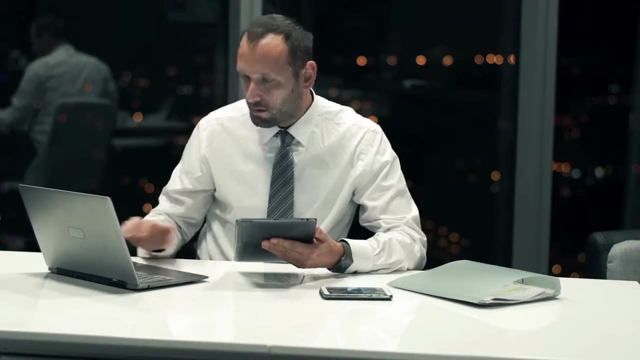 In order for two or more transceiver modules to communicate with each other, they need to be on the same channel. This channel could be any frequency in the 2.4 gigahertz ISM band. Now, such transceiver modules could be a variety of things, such as a laptop, a smartphone. 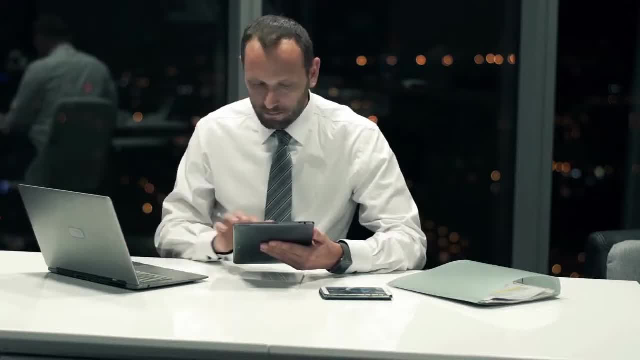 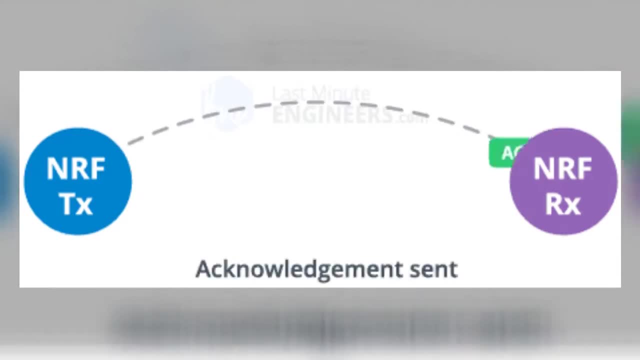 or your internet modem. Now let's take a look at a mini-example. Here we have two modules: one TX, meaning transmitter, and one RX, meaning receiver. When the data is sent, the receiver will automatically send the data to the transceiver module. 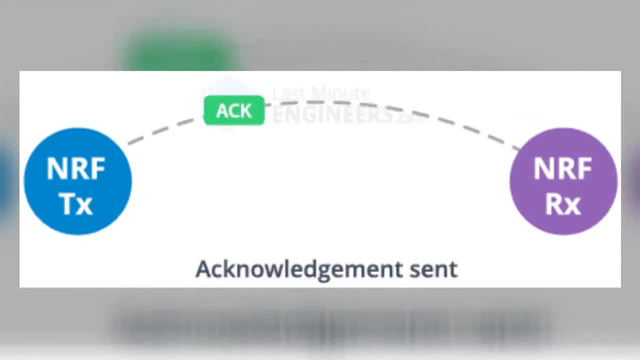 The receiver will automatically acknowledge the data and tell the transmitter about it. Now, this doesn't just have to be two NRF modules. It could even be a smartphone communicating with the module. It uses the same principle. The transmitter will send some sort of data over a specific frequency, known as a channel. 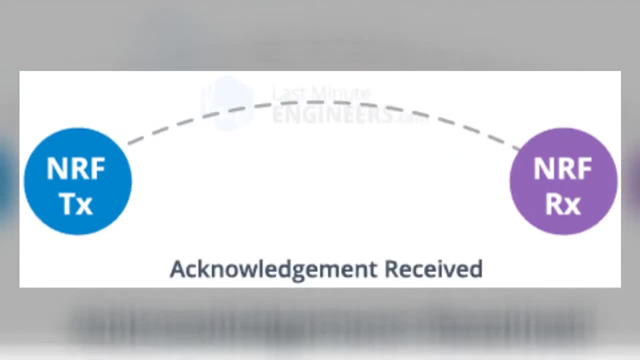 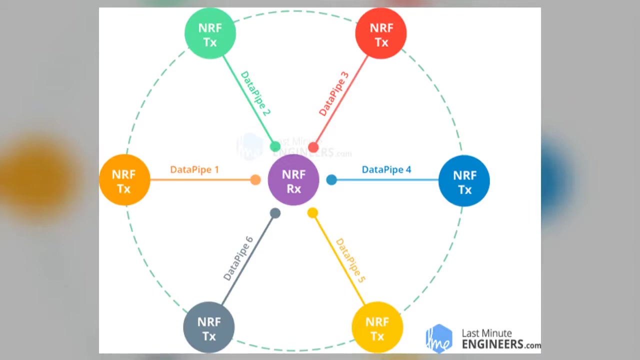 If the receiver is listening on that same channel, it will receive the data and automatically acknowledge the transmitter. Now the roles of these two modules could swap, And one could transmit the data to the other. Let's move on to a very important topic. 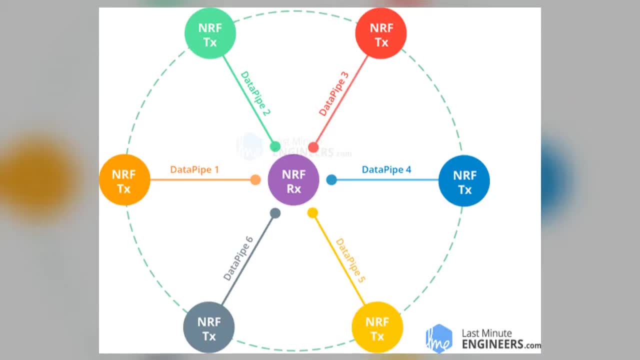 Each channel occupies a bandwidth of less than 1 mHz. This gives us 125 possible channels with 1 mHz spacing, So the module can use 125 different channels, which give a possibility to have a network of 125 independently working modules. 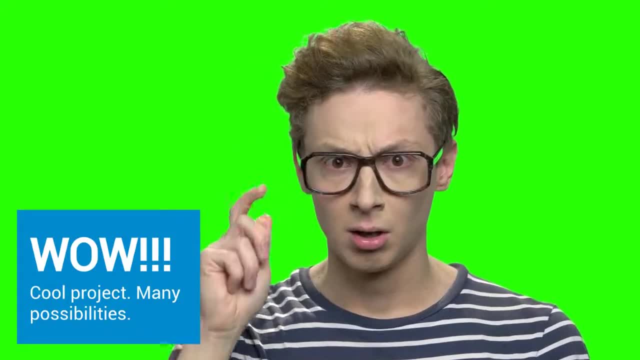 This allows us to hook up many of these together And have a network of 125 independently working modules. This allows us to hook up many of these together And have them all communicating with each other. Now let's switch gears to discuss Bluetooth. 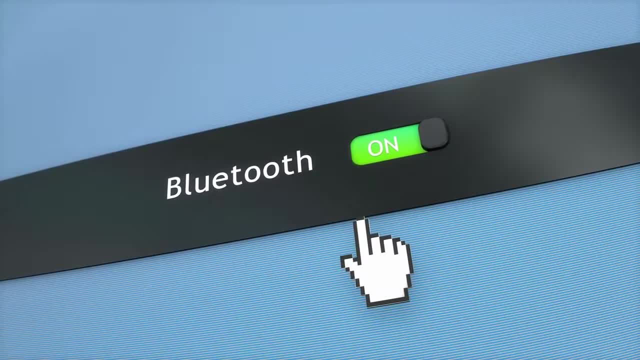 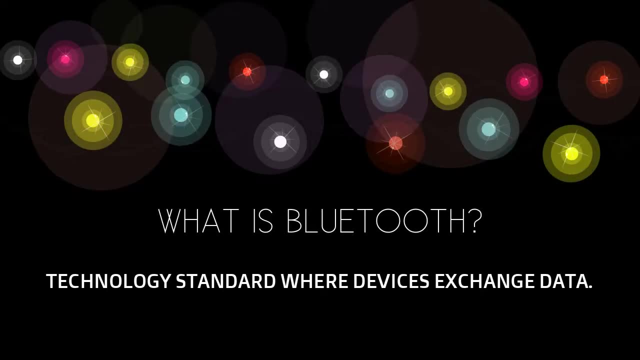 What could this module have to do with Bluetooth, you ask? Well, first let's define Bluetooth. It's a standard technology in which two devices bond or pair with each other to transmit and receive data. Very similar to the concepts we just discussed. 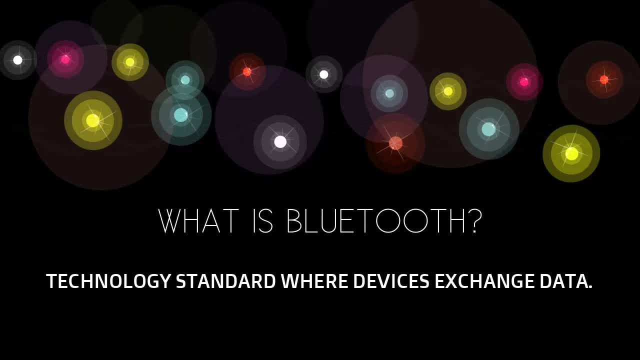 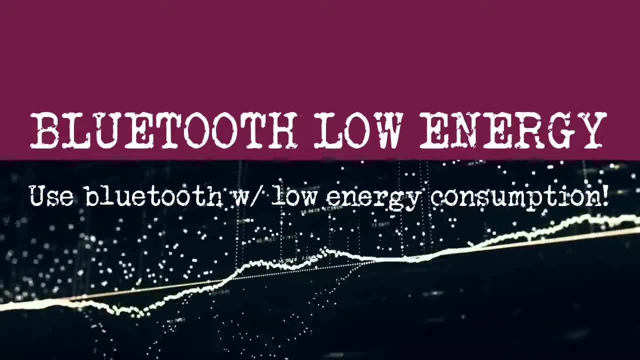 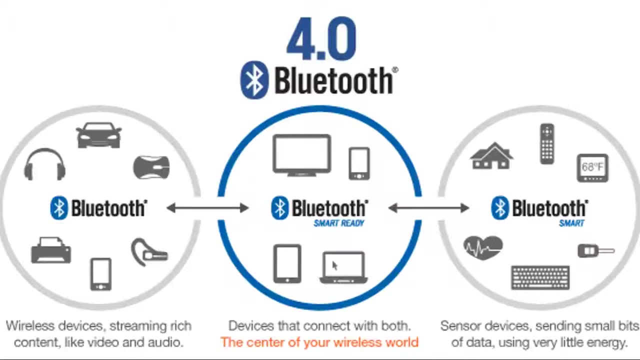 Bluetooth Low Energy, also known as BLE, allows devices to consume low-energy data. BLE has been used in novel applications such as healthcare, fitness beacons and security. Developers have created libraries that one can use in conjunction with the Arduino to transmit and receive data on the NRF24L01 using Bluetooth Low Energy technology.